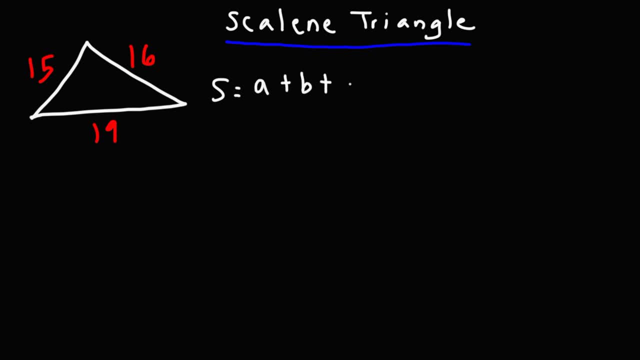 First we need to find s. s is one half of the sum of all three sides, So basically s is one half of the perimeter. Once we know the value of s, we can plug it into this formula to get the area of the scaling triangle. 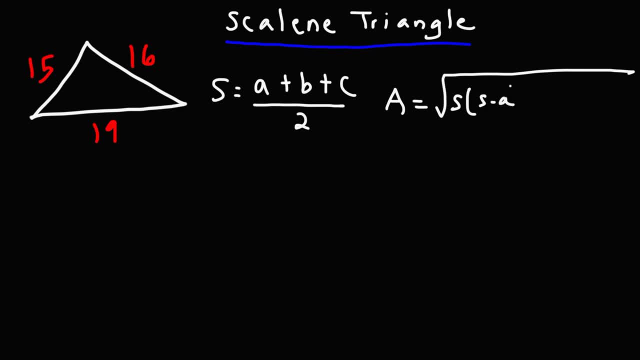 So it's the square root of s times s minus a, times s minus b, times s minus c. So let's say that a is 15.. We're going to say that b is 16 and c is 19.. It doesn't really matter the order in which you assign them, so you'll still get the same answer. 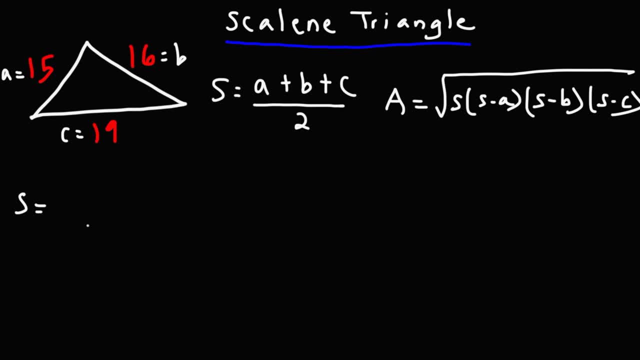 Now let's calculate one half of the perimeter. So this is going to be 15 plus 16 plus 19 divided by 2.. 15 plus 16 is 31.. 31 plus 19 is 25.. No, that's 50.. 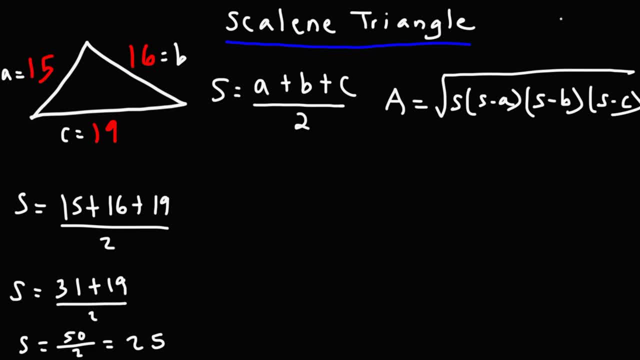 50 divided by 2 is 25.. I automatically jump to the final answer. So s is 25 in this problem. Now let's calculate the area using the second formula. So we have s minus a 25 minus 15.. 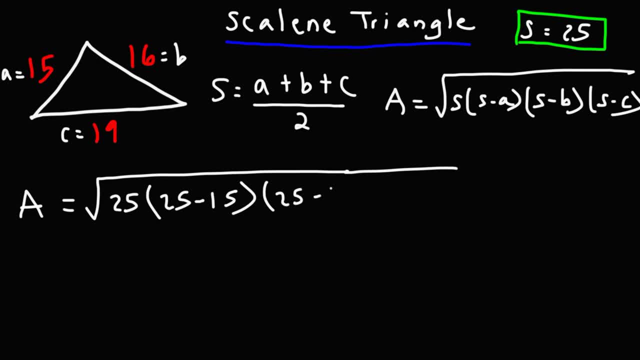 And then s minus b, 25 minus 16. And s minus c, 25 minus 16.. 19.. 25 minus 15 is 10.. 25 minus 16 is 9. And 25 minus 19 is 6.. 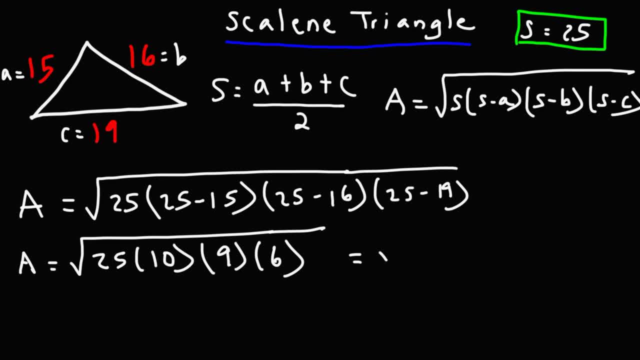 So what I like to do is I like to take out the perfect squares. 25 is a perfect square, 9 is a perfect square, And we're left with 10 and 6.. But 10, I'm going to break that into 5 and 2..